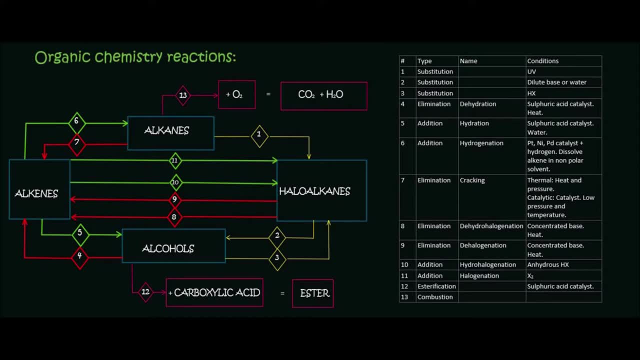 13 main reactions that you need to know, and here they are, staring right back at you. What we're going to do in the next couple of videos is we're going to go through each of them one by one, and I'm going to help you to familiarize yourselves with them, and so you'll see that it's just they're. 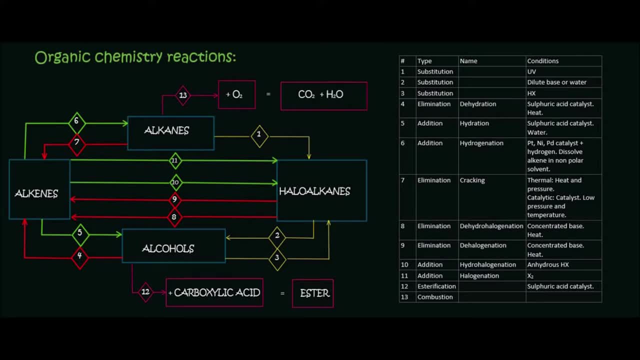 going to, you'll see how easy they actually are. So in this lesson we are most likely going to: well, we're definitely going to do reaction number one and then, if there's time, we will also do reaction number two. So, reaction number one: if we look at the diagram, we start with an alkane. Now you know. 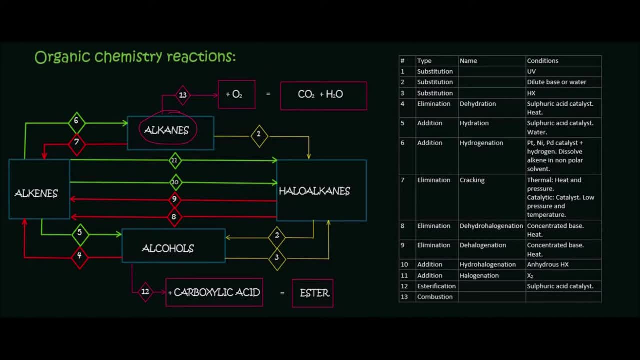 what an alkane is. it's got the carbon and hydrogen single bonds and we somehow going to convert it into a hydrogen. So we're going to go with a halo alkane. So a halo alkane is when you have a halogen. Now, if we look at our table, 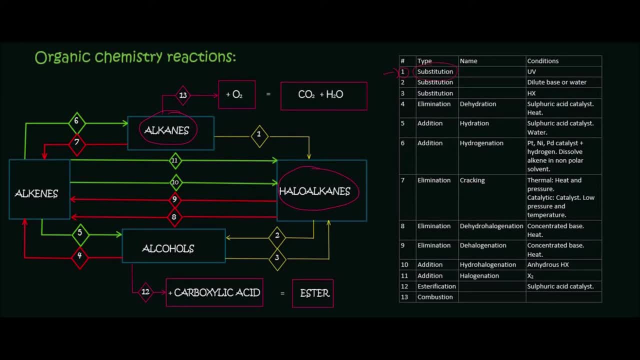 reaction number one is called substitution. I will explain that just now, and the conditions that we're going to need for this reaction is going to be UV light, So you're typically going to have to do this outdoors in the sun. but I'm going to explain everything now. So we're still busy introducing. 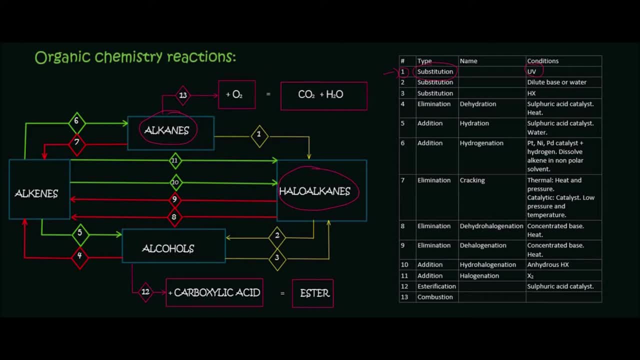 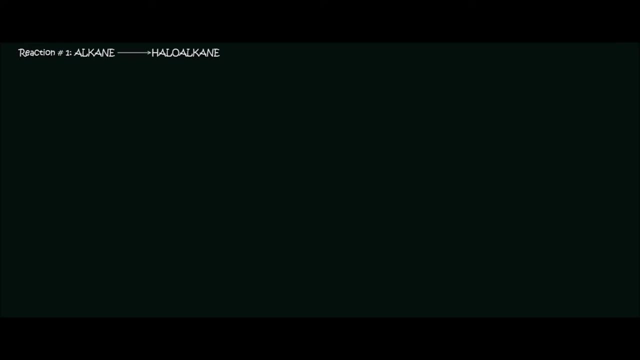 this idea. So we're going to go with an alkane to a halo alkane. So although that table looked- or that diagram probably looks- very overwhelming, we're just going to take it in baby steps. Of course we can't learn it all looking at it all like in one picture. 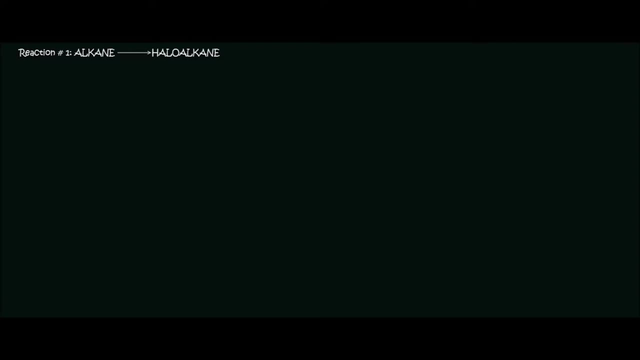 but that picture is what we're going to use as our reference, and it's also going to be a good thing to know when you're in your exams. So we're going to start off with an alkane and we're going to turn it into a halo alkane. 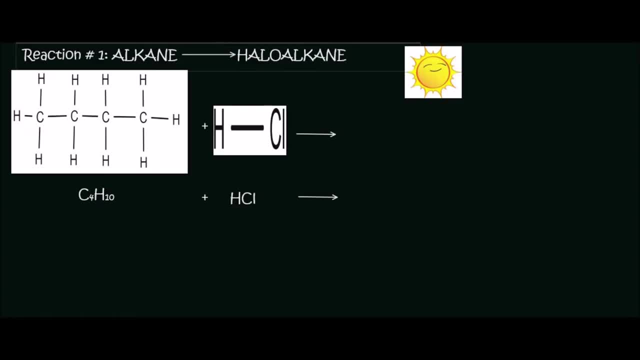 So let me bring out an alkane. So there we have our alkane, which is butane, which is C4H10. then we're going to add some HCO to that and we said that the product is going to be a halo alkane. 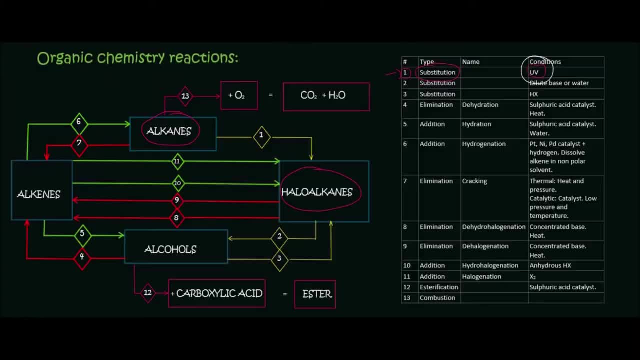 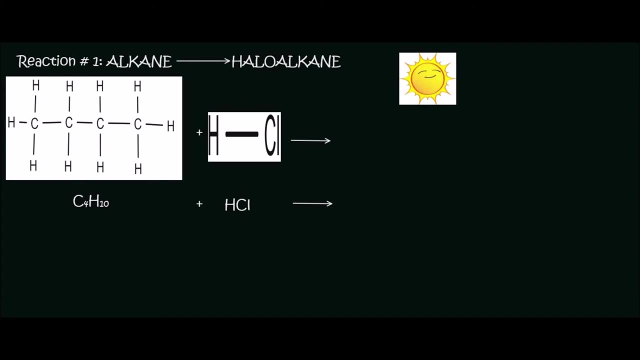 And then remember, if you look on the table over here, we could see that we needed some UV energy, and that's why I've got the sun in the picture. And so what's going to happen is it's a substitution reaction. So all that happens is that this Cl- you can imagine that it will just switch place. 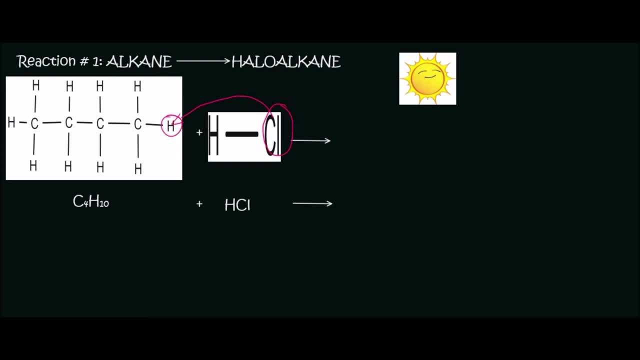 with this H over here, And that's all that happens. Why it happens, we don't need to know, We just need to know that it happens. okay, So your product then is going to be the following: And so here we can see that the H and the Cl have switched places. And so what would our other 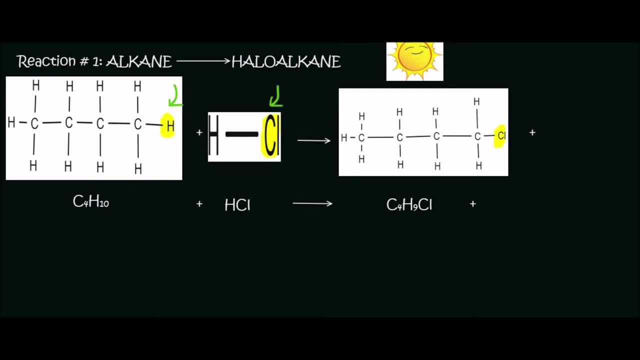 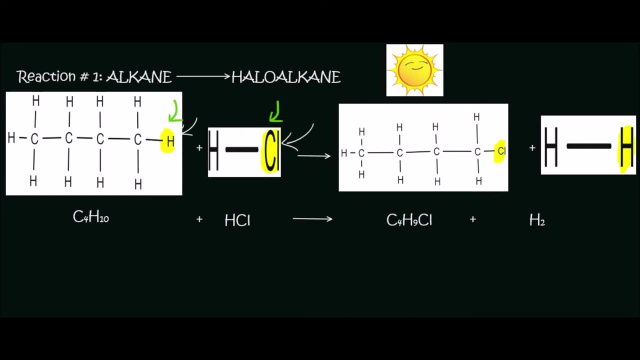 product be Well, well done if you realize that it's going to be the following: We're obviously going to be left off with hydrogen, because this H over here gets replaced by this Cl, And so we can see the Cl lands up over here, And so this H. let's go this way around. 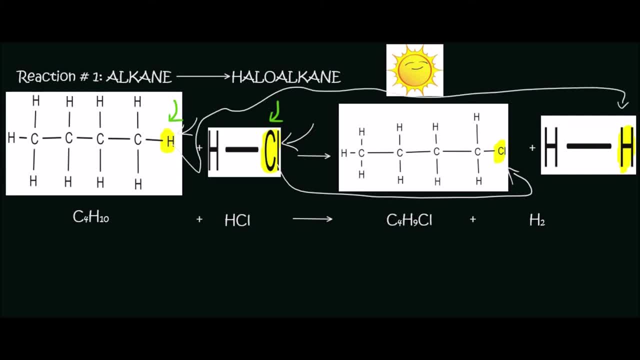 ends up over there. So, guys, I'm going to stop there, just so you have a nice introduction to the way the reactions are going to work. This is called a substitution reaction, because you substitute means to replace, So we replaced this with that. That is all you need to know. 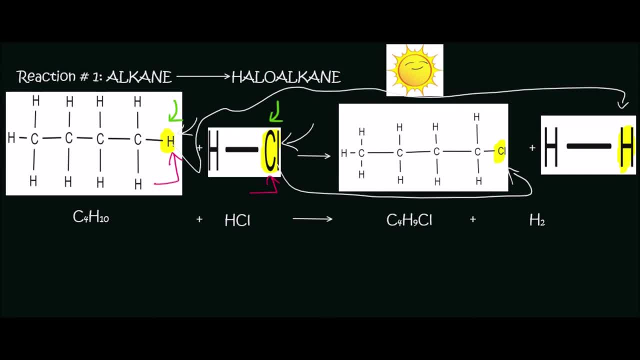 So now an alkane can be turned into a halo alkane by using substitution, And the way to do it is to make use of UV energy, And that's why I drew the sun. So there's 13 types of reactions that we are. 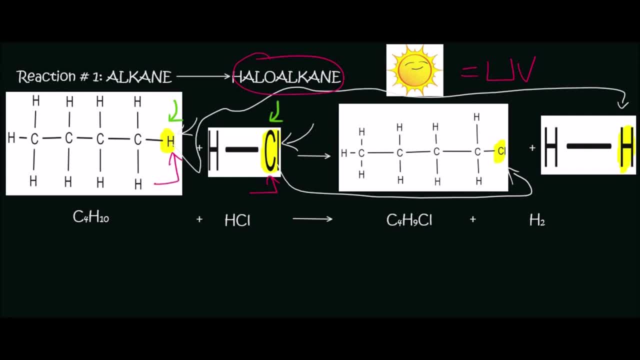 going to look at, But they all follow this type of structure where they'll all make sense. Trust me, as we go through each of them, you'll see that it all makes sense. Thank you for watching.